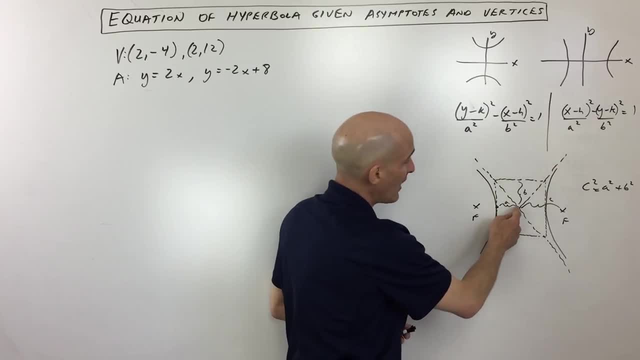 recognize is that when you have these asymptotes, you know the slope of a line is the rise over the run. okay, so you can see, you can figure out. well, if I go this much for the rise, this much for the run, in this case it's going to be B over a, okay, but you can see that the distance from the center to 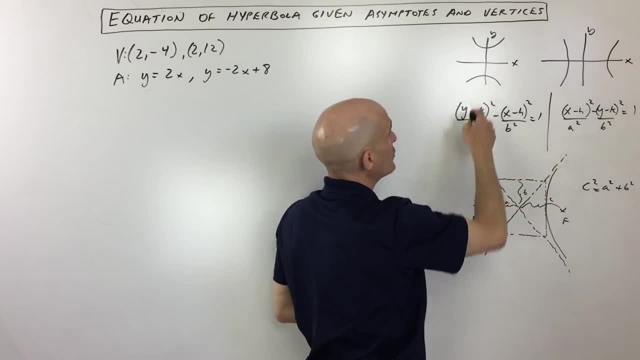 the left to the right is going to be A over A. so only if that's not the case, you're not even going to have the difference between A and B, so you can see that the slope of the line is going to be B over A. okay, but if it was opened the other direction, like so, you would actually be doing A. 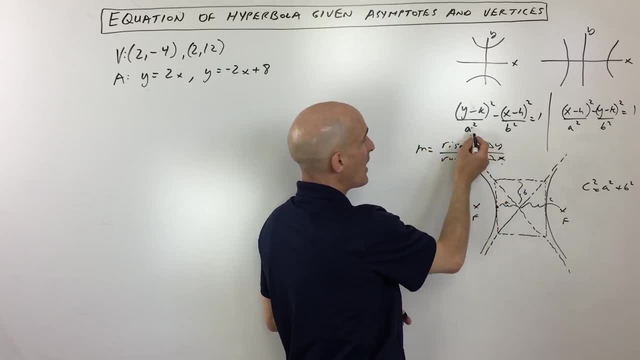 over B. so an easy way to remember this is that you know, when you think of the slope, slope is what it's: the rise over the run, which is really like the change in Y over the change in X, right, and when you think about the change in Y, this number here, that's underneath the Y, is going to be your. 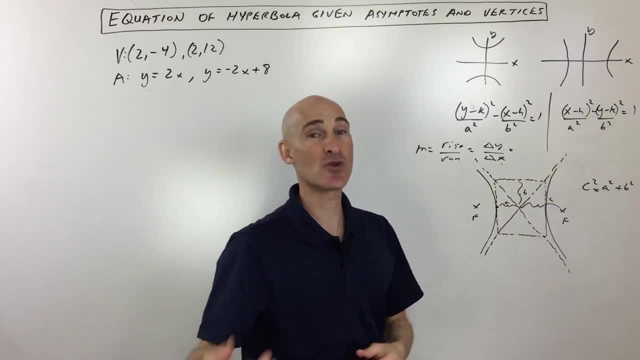 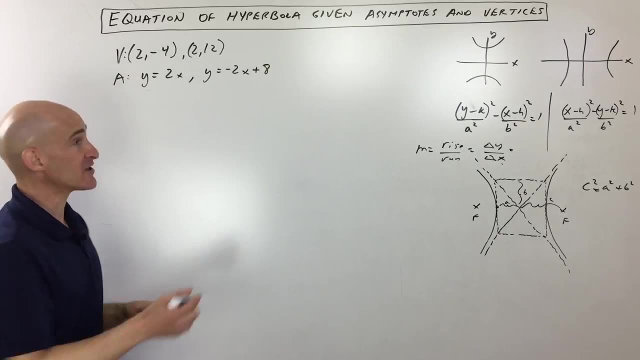 So it's easy to remember: the number underneath the y is the rise, the number underneath the x is the run when you're calculating the slope for your asymptotes. But let's get into this example here. So what I always like to do is I like to draw a sketch just to see what I'm dealing with, to help me to formulate my equation. 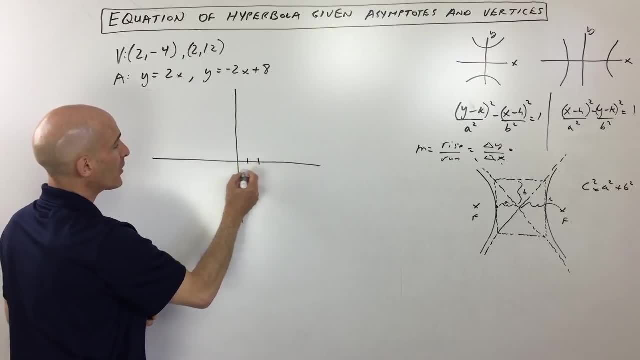 And you can see that the vertices here that they give us are at 2, negative 4, 1, 2, 3, 4, so 2, negative, 4 right about there and 2, 12.. 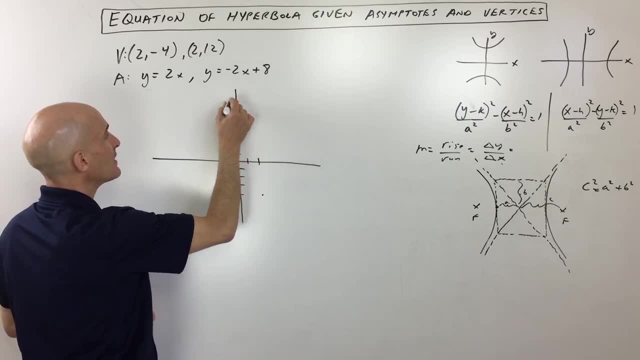 Okay. so let's see 1,, 2,, 3,, 4,, 5,, 6,, 7,, 8,, 9,, 10,, 11,, 12, way up here, right, Okay, so that's our other vertex. 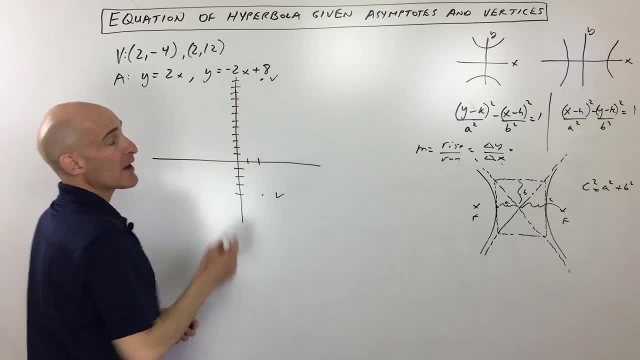 And then the asymptotes are at: y equals 2x and y equals negative 2x plus 8.. Okay, first thing I want to do, though, is I want to find the center point, And the center point is going to be halfway in between those vertices. 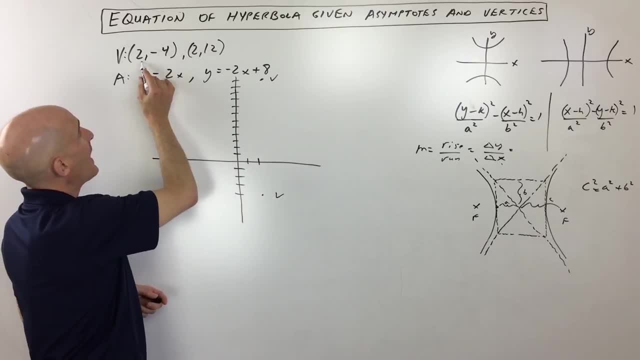 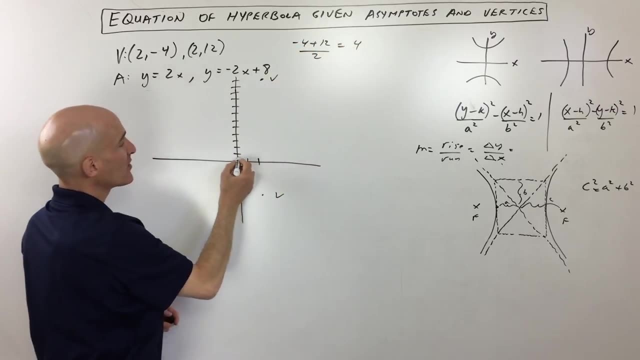 So we can either count and find the midpoint, or you can take negative 4 plus 12, okay, add those together and divide by 2.. So that's going to come out to 4.. So we're really over here at 2, 4, which is going to be right there. 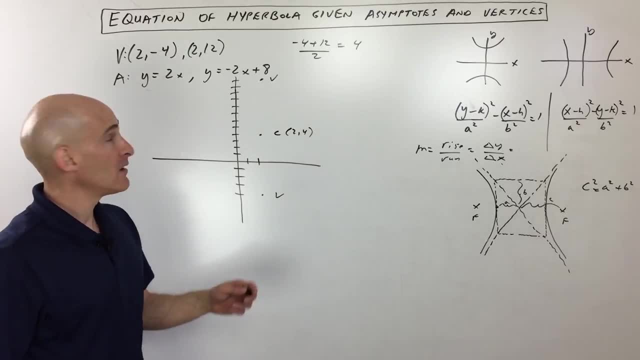 Okay, there's our center Center 2, 4.. Okay, then, from the asymptote perspective we've got y equals 2x, So that means it's going up 2 over 1, like this okay. 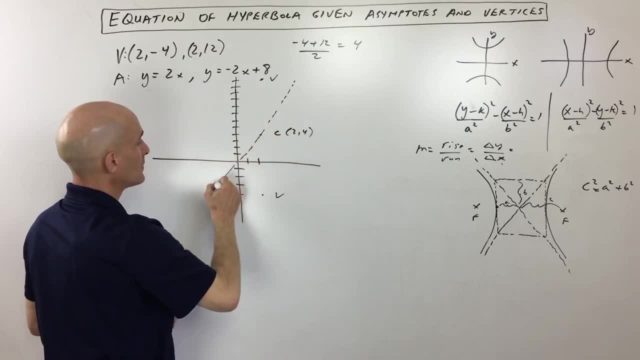 And so you can see it's looking something like this. And then for the next one, y equals negative 2x plus 8.. So 2,, 3,, 4,, 5,, 6,, 7,, 8.. 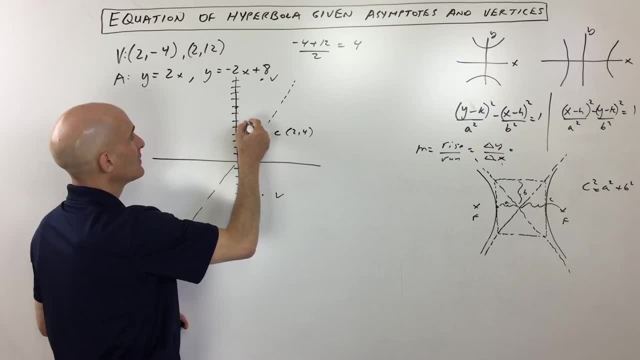 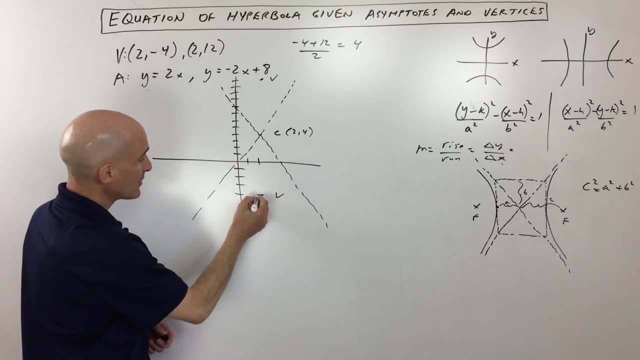 And this one has a slope of negative 2, okay, like so, Okay, approximately right. And then we know that the hyperbolic, Okay, It's closer and closer to those asymptotes. So I'm just drawing a quick sketch here for us so we can see. you know that it's opening up and down. 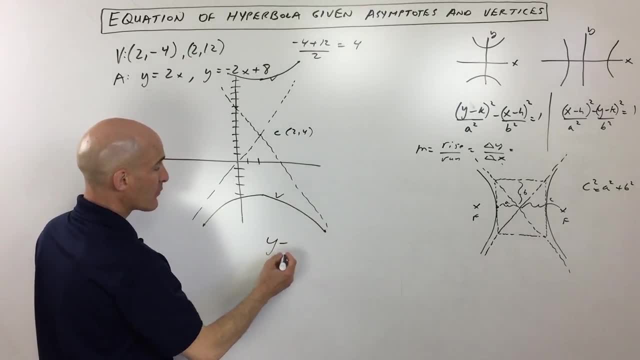 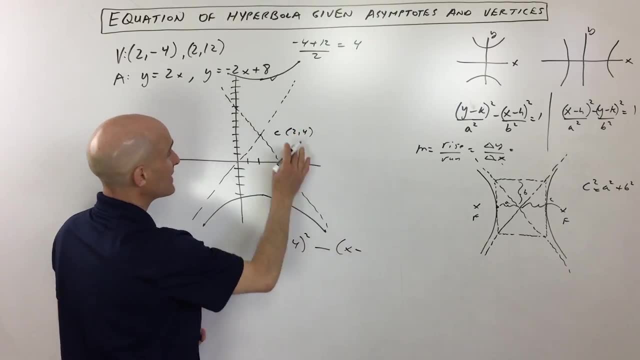 So we know it's opening up and down. So that means that we're going to be looking at hyperbola in this form. It's going to be y minus the y-coordinate of the center squared minus x minus the x-coordinate of the center squared equals 1.. 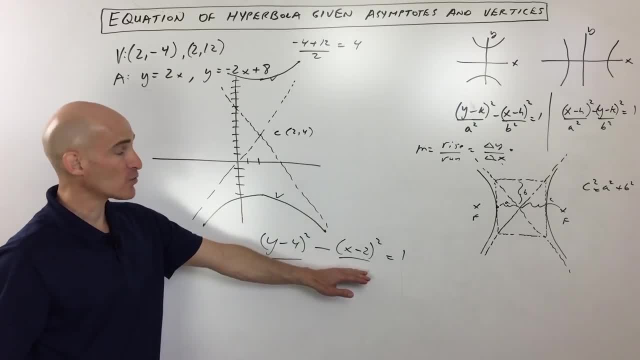 And now what we have to do is find these denominators. We need to find our a squared and our b squared. Well, remember the distance from the center to the vertex. this distance right here is a, And we can see that. that is how much. 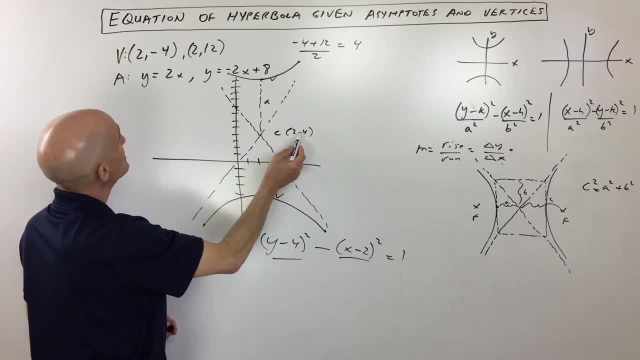 Well, let's see That's going to be 8 units. So you can see, this is the difference between 4 and 12.. So that's going to be 8 squared, which is 64.. Okay, so that's our a squared. 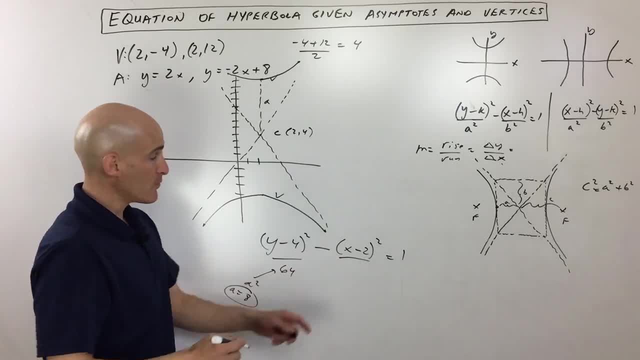 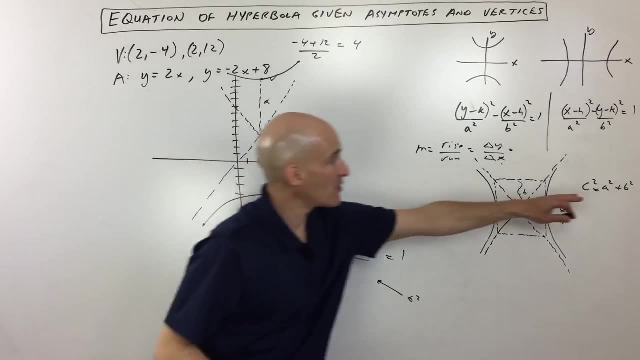 And we figured out that a is equal to 8.. Now all we have to do is find our b squared. Okay, that's this value right here, And the equation that relates all those together is: c squared equals a squared plus b squared. 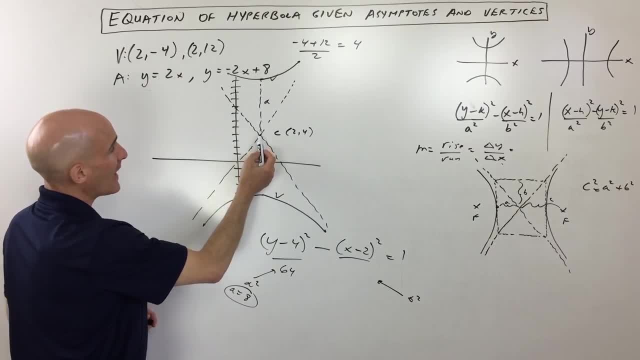 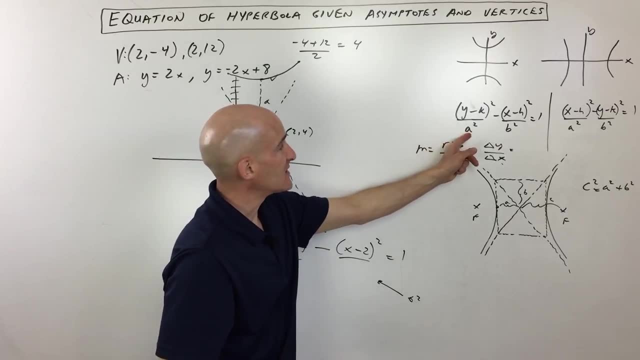 And we also know that the slope of this asymptote here is going to be the rise over the run. Okay, so when we think about the rise over the run we can think about in this case: a divided by b is our slope. 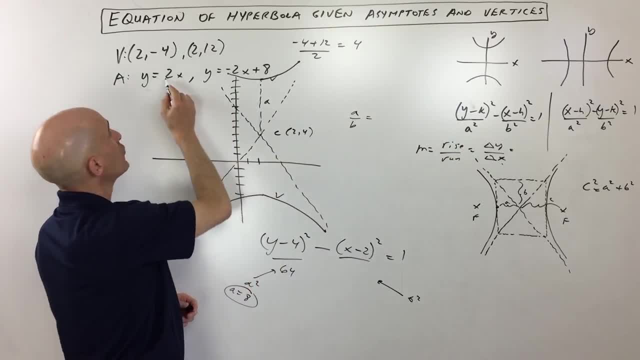 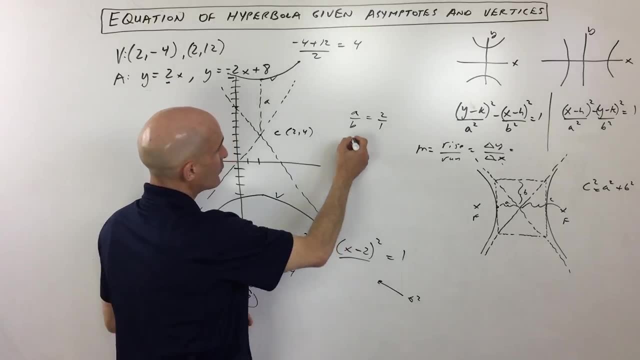 So let's write that down. So a divided by b is equal to our slope, And we know the slope is 2, right? So that means we're going up 2 over 1.. So that means that. let's see, what do we have here? 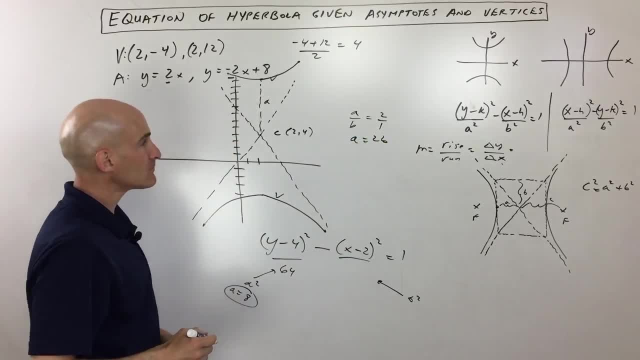 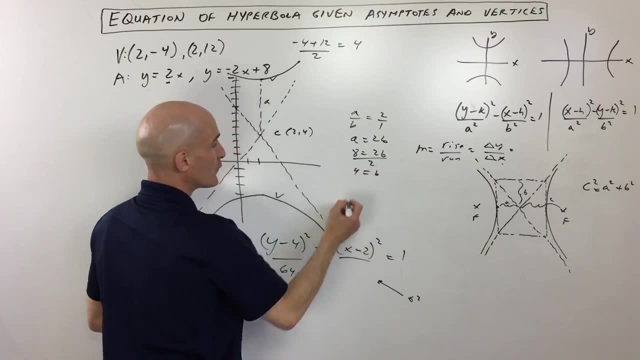 We have a is equal to 2b, right, And we know that a is 8. So 8 equals 2b divided by 2. And you can see that b is equal to 4. But in our equation we want b squared. 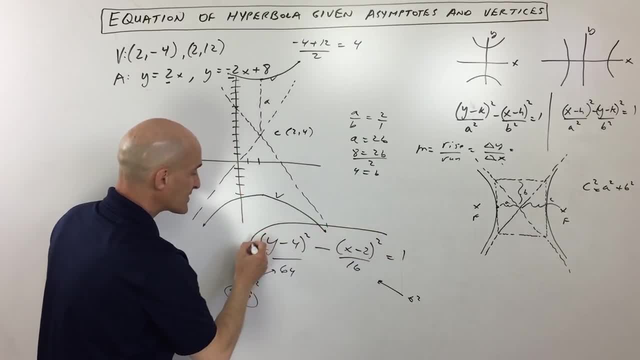 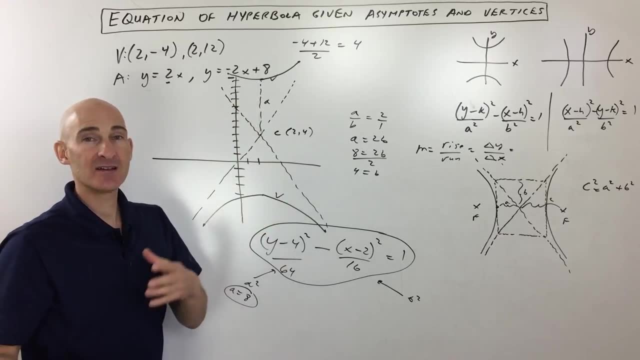 So this is going to be 4 squared, which is 16.. And there we go. That's the equation of our hyperbola. given the asymptotes and the vertices, What I like to do is just sketch it out so I can kind of take a look at it as I'm working through it.